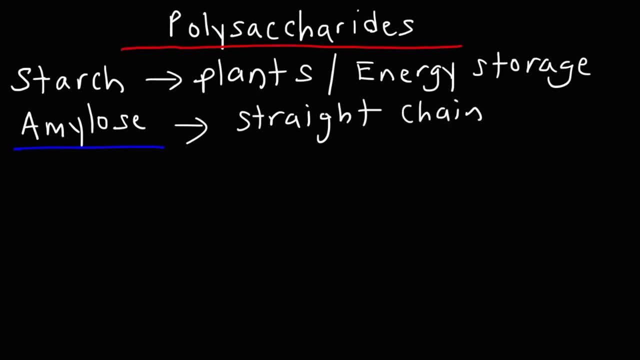 of glucose monomers. So amylose would look like this: It would connect all of the glucose monomers in a straight chain. Now the bond that connects the glucose monomers is an alpha-1,4-glycosidic bond. 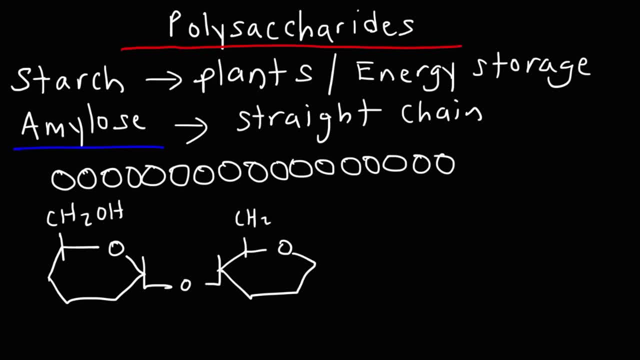 So I'm not going to draw the entire glucose monomer, but I just want to show you why it's called an alpha-1,4-glycosidic bond. So this is carbon-1 of the first glucose unit on the left. 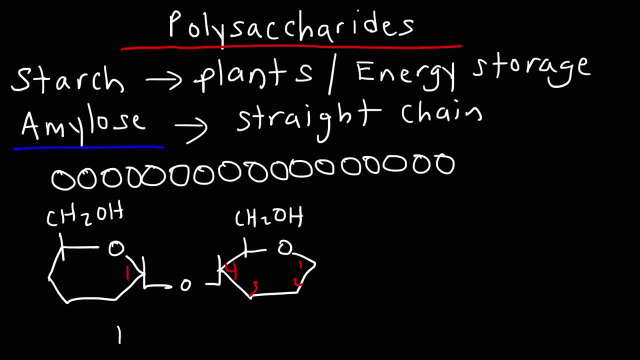 and here we have carbon-4.. So it's a 1,4 bond. Now you need to be familiar with the alpha and the beta forms of glucose. In the alpha form, the OH group on carbon-1, it's facing the downward. 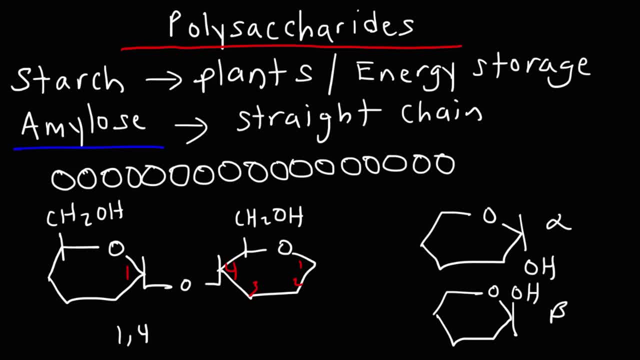 direction. The beta form of glucose has the OH group pointed up. So, as you can see, this is the alpha form. So thus we have an alpha-1,4-glycosidic bond. So amylose only has this type of glycosidic bond. 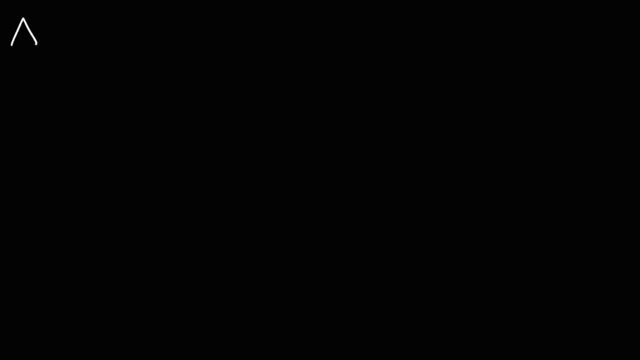 Amylopectin is different. Amylopectin contains branch structures, So it still has a straight chain, but occasionally you'll have chains that will branch off from the main chain, So that will be an example of amylopectin. 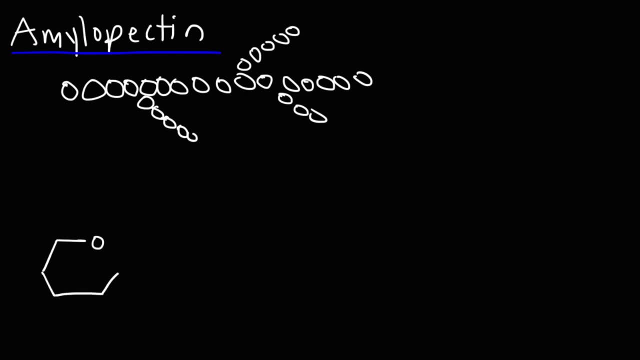 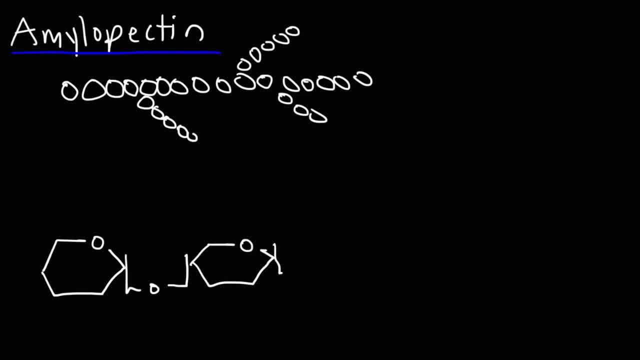 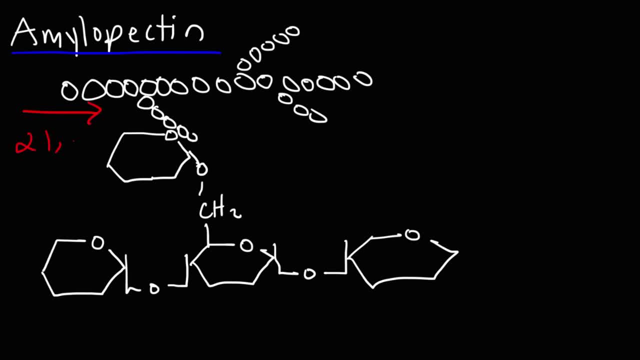 So the straight-chain part of amylopectin has the alpha-1,4 bond, as you can see here, But now the branch part of amylopectin has an alpha-1,6 bond. So this is carbon-1,2,3,4,5,6.. 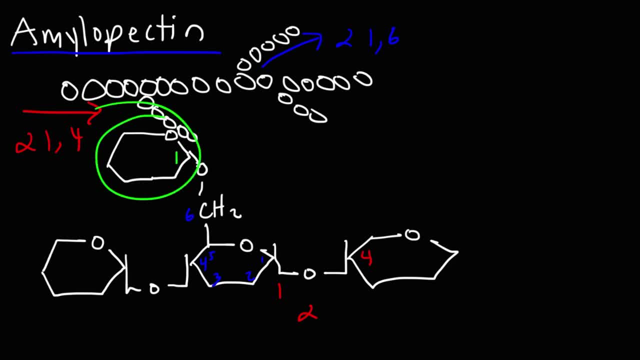 And that's connected to carbon-1 of this sugar unit And this is still an alpha bond. So amylopectin contains an alpha-1,4-glycosidic bond. So this contains two types of glycosidic bonds. 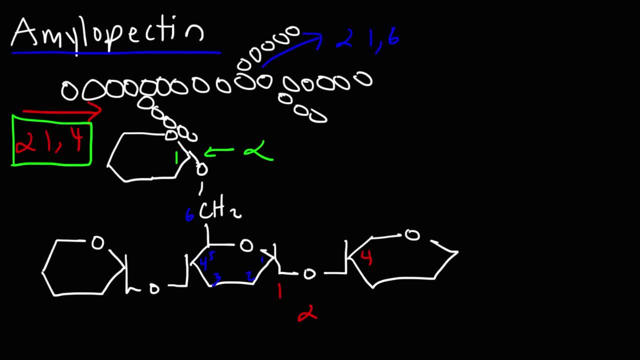 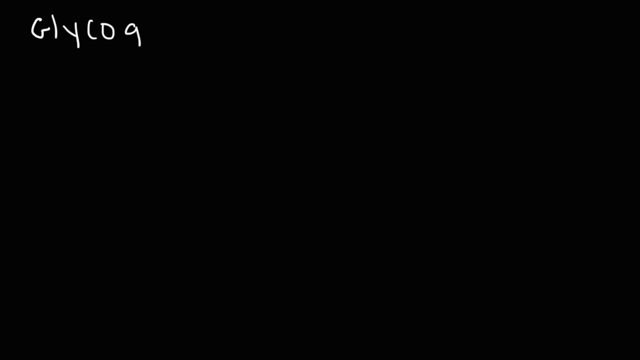 The alpha-1,4,, which is responsible for the straight-chain part of amylopectin, And the alpha-1,6-glycosidic bond, which is responsible for the branching that we see in amylopectin. Now, the next type of polysaccharide that we need to talk about is glycogen. 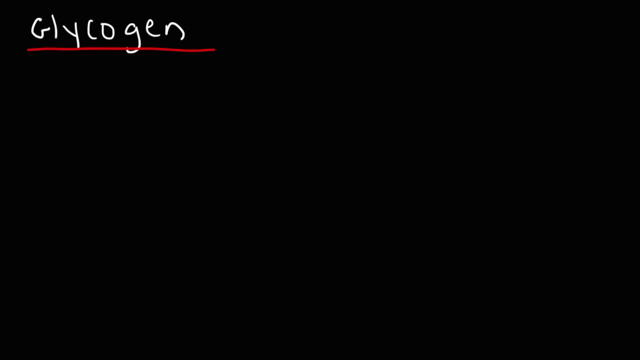 Glycogen is a polysaccharide that is made up of glucose monomers. Now we said that starch is here. Glycogen is found in plants. A good example of starch will be potatoes. Glycogen is the starch that is found in animals. 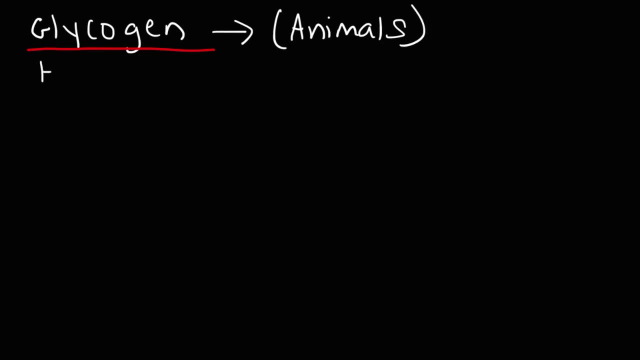 Now, glycogen is highly branched. Like amylopectin, glycogen has alpha-1,4-glycosidic bonds And the alpha-1,6-glycosidic bonds, which are responsible for branching. The next type of polysaccharide that we need to talk about is cellulose.